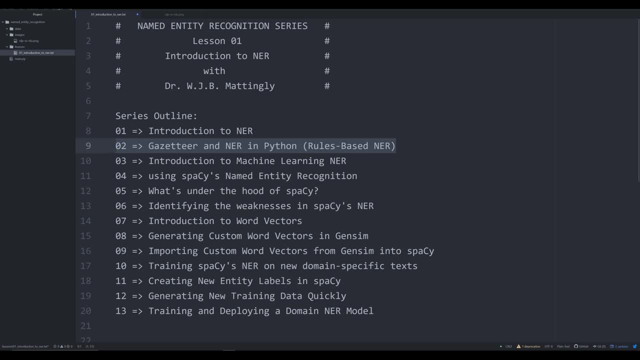 I'll talk about in just a second. The reason for that shift is because of the way in which machine learning can generalize on unseen data or unseen texts. However, rules based any are is still very useful for very specific problems And in order to understand when. 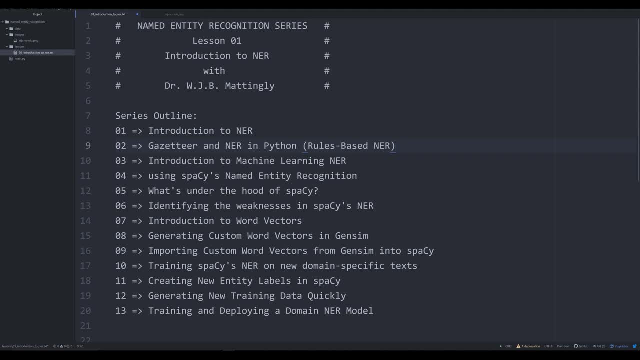 you should use machine learning, any are. it's important to understand what other options are out there And also- this will show us in this video, video number two, why rules based methods are not necessarily the right solution for a lot of different any are problems. 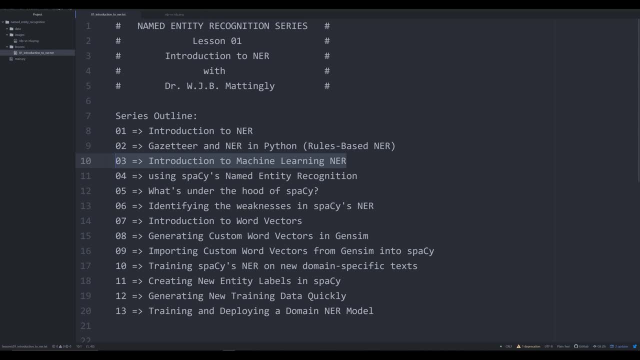 And the next video, number three, I'm going to be introducing you to machine learning- any are, And kind of some of the basics. If you've never ever heard of machine learning or used machine learning, Don't worry, I'm going to presume no knowledge on the part of the listener. 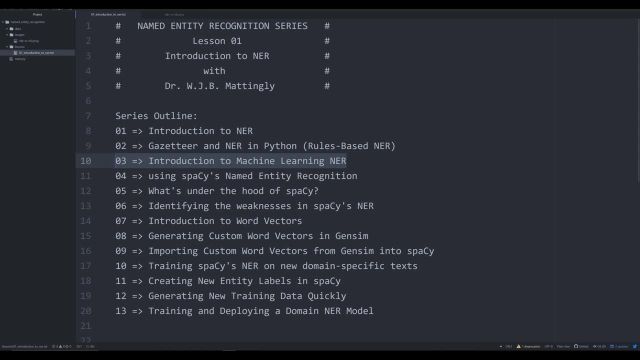 or viewer. And if you want to learn more in depth about machine learning, I have a whole series on machine learning for the Digital Humanities. In this video I'm just gonna kind of run over the basics very quickly, just the core stuff that you need to know. 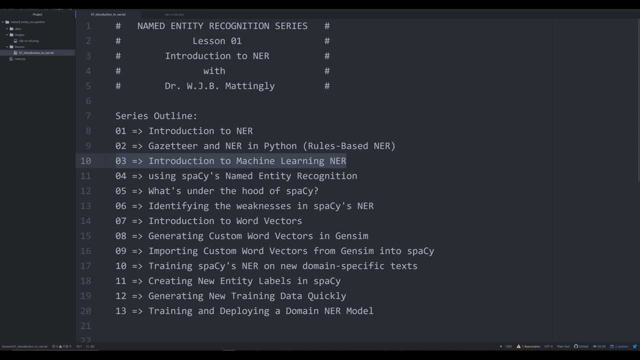 in order to use Python machine learning libraries that rely on machine learning practices, And the one that we're going to be using in the is spaCy. I'm going to talk a lot about spaCy when I'm done going over the series outline. 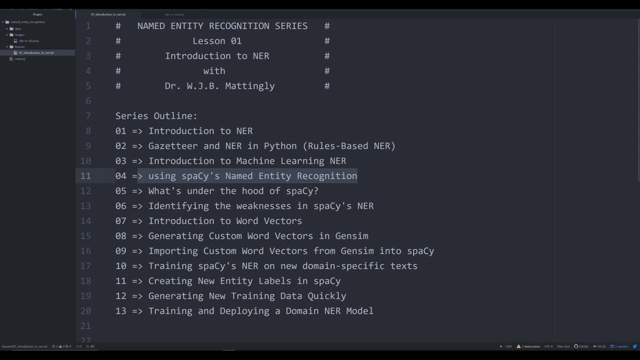 spaCy is a state-of-the-art commercial NLP software, so natural language processing framework, And one of the pipelines that it has is an NER pipeline. Now it's very, very good at performing general named entity recognition And in order to understand how, 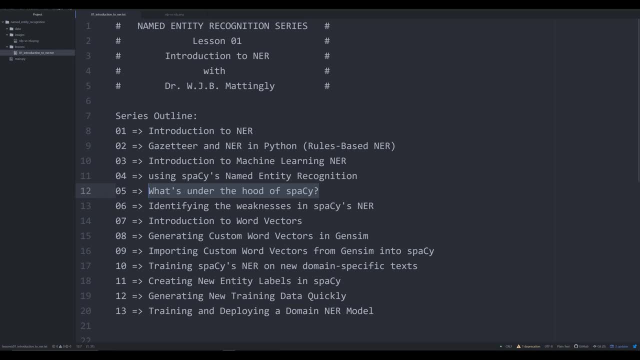 spaCy works and why it's good at what it does. in video five we're going to look under the hood of spaCy, see what makes it tick and see what makes a machine learning model actually work and what the pipeline looks in its directory. In video number six we're going to do probably the 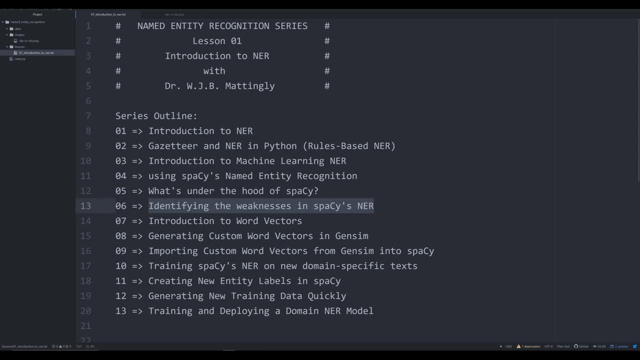 most important thing in this whole series: We are going to identify the weaknesses in spaCy's NER model. Now, this is not a criticism of spaCy- not at all. Explosion AI, who made spaCy, is a fantastic company and they have produced state-of-the-art models that they make available. 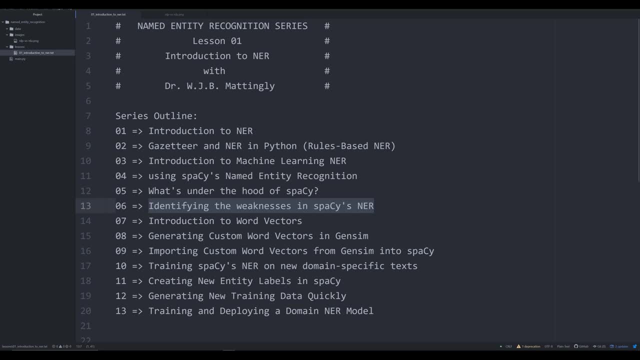 to the general public. This is a criticism of machine learning, natural language processing in general, and it shows the difficulties of performing the task And it's going to come down to what we call domain ambiguity or domain problems. In other words, a lot of machine learning models like spaCy's are trained. 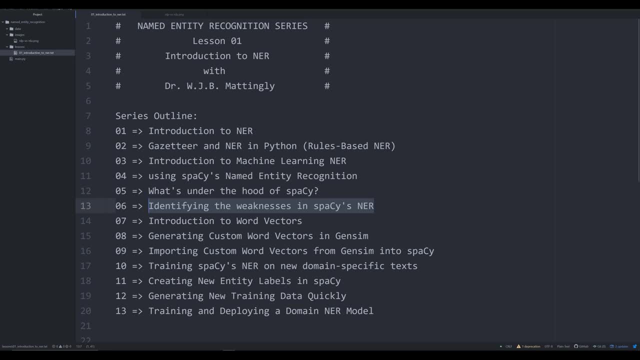 on a general web dataset, a general corpus from a few different areas of the web. However, when it comes to using that on something that is very specific, such as law, healthcare, holocaust, South African history, you'll find that the spaCy model doesn't perform. 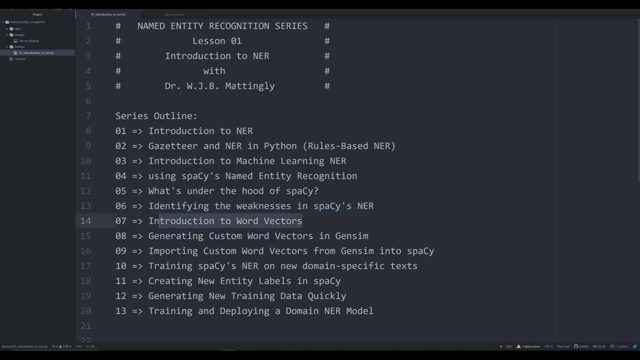 very well, And we're going to look at those weaknesses in video six And then for the rest of the series, I'm going to show you how to overcome those problems through a few simple steps that can be a little daunting. if you don't know how to do them, I'm going to break them down. 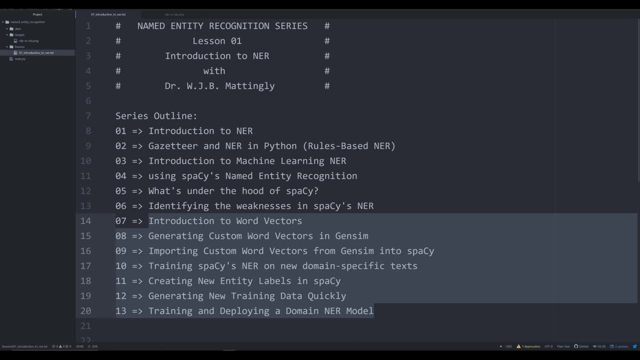 into very easy-to-understand steps and provide you with the code and solutions for solving those problems, so that you can use NER on any set of corpora that you might have, Whether it be documents from the holocaust, documents from US government, whatever. 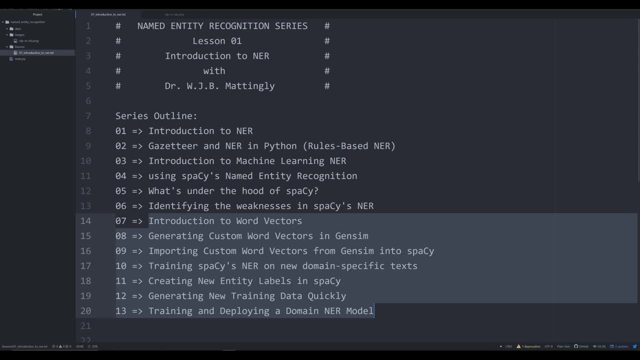 it doesn't matter. I'm going to show you how to train a custom model to perform much better on your data. And if you've used spaCy's NER and you've seen bad and inconsistent results in your data, then these steps are going to show you how to solve that problem, And we're going to break. 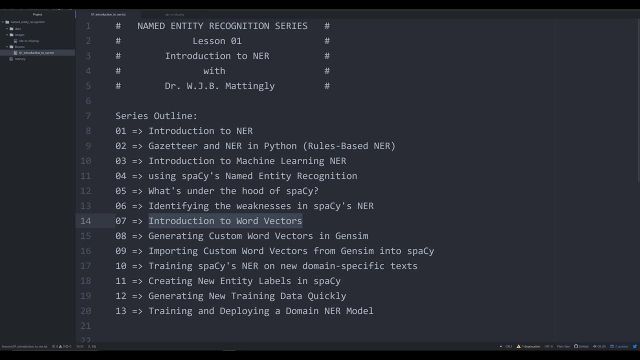 this down by introducing you to something called word vectors. If you don't know what those are, now you will definitely know what they are. I'm going to explain all that in layman terms in video seven. Then we're going to go into showing. 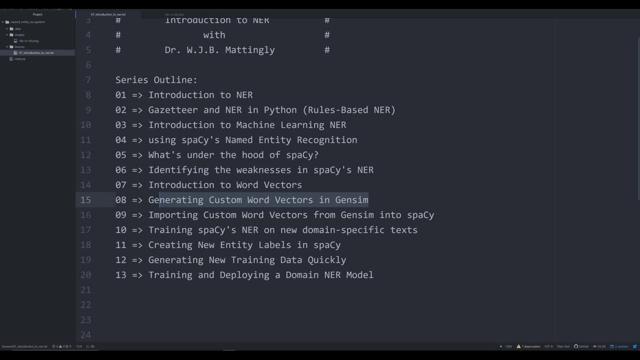 you how to generate your own custom word vectors using the Python library Gensim. This is going to be very important so that in number nine, we're going to show you how to inject and import those custom word vectors into spaCy, which is going to increase your. 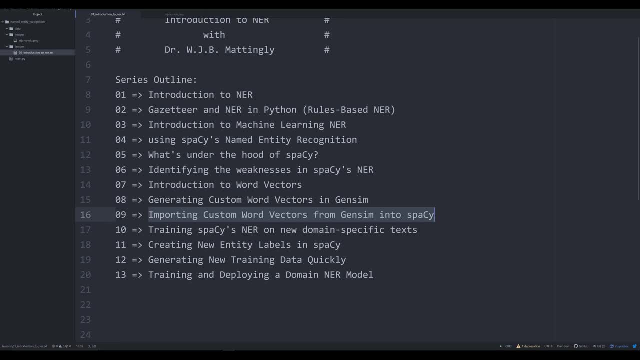 accuracy of NER substantially, even without training. However, training is important in machine learning. You need to train the spaCy model and I'm going to show you how to do that in video 10.. In video 11, we are going to start creating new entity labels in spaCy. 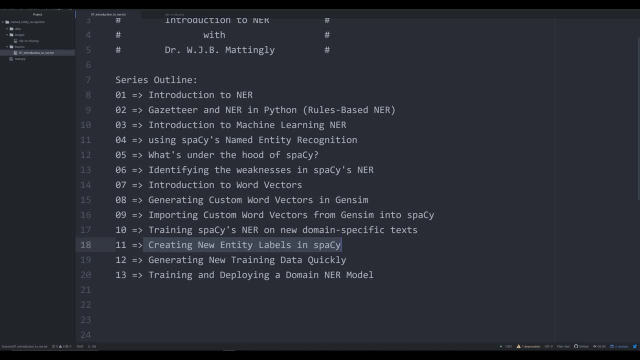 So, if you're looking at a corpus of texts that are important to your research, the 18 named labels in spaCy might not they might be applicable to your research, but there might be other labels that you want to assign. So, if you look at the Holocaust, like I do, some labels that you might 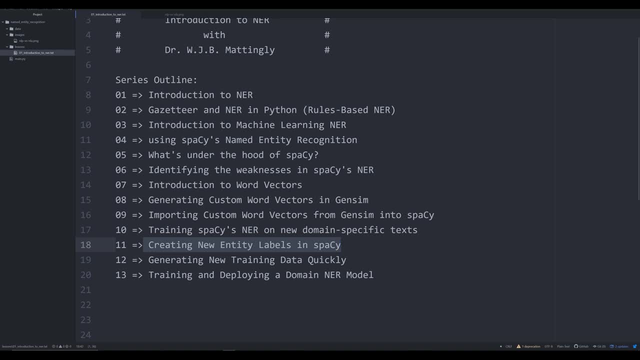 want to assign to entities in a text might be things like concentration camps, ghettos, et cetera. I'm going to show you how to create new labels in spaCy and train models on those new labels. And then, in video 12, I'm going to show you how to quickly and easily generate a lot of. 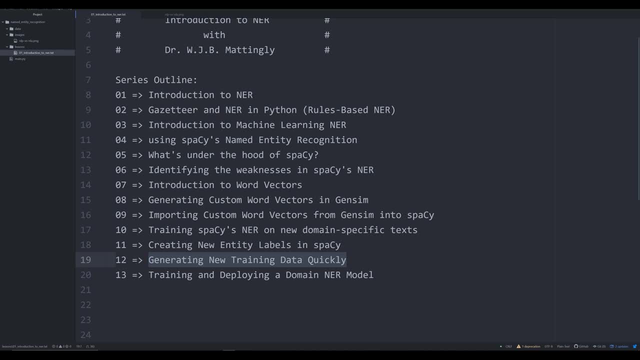 training data that you can easily manually check. It's going to be a few simple tricks and tips that allow for you to do this process quickly so that you can cultivate a large training set that you can then, in video 13,, I'll show you how to do this. You can then use to train a new spaCy NER. 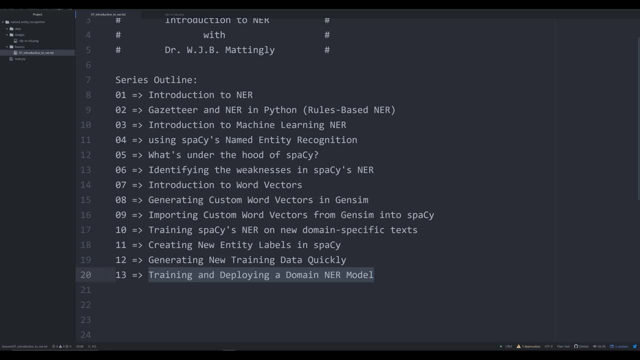 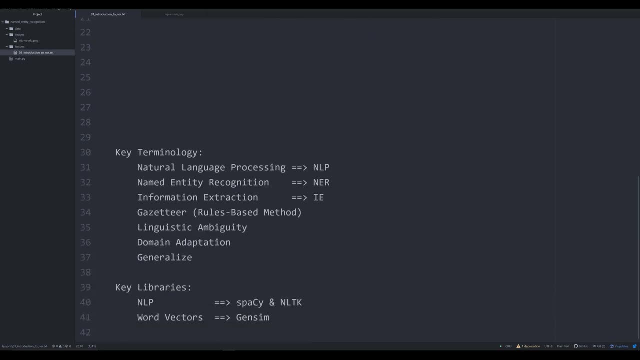 model. I'm going to show you how to do that and then have something that you can be proud of, something that is actually deployable on a whole bunch of unseen data. So that's kind of the general course outline, Some of the key terminology. 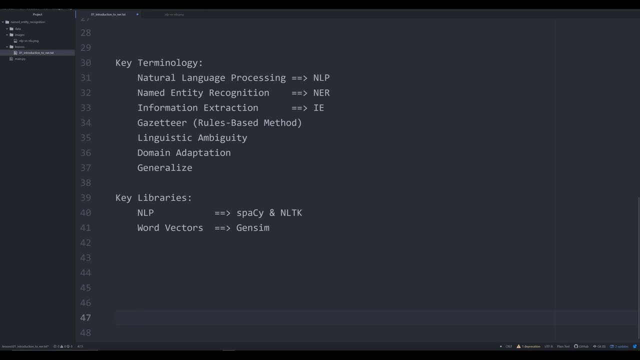 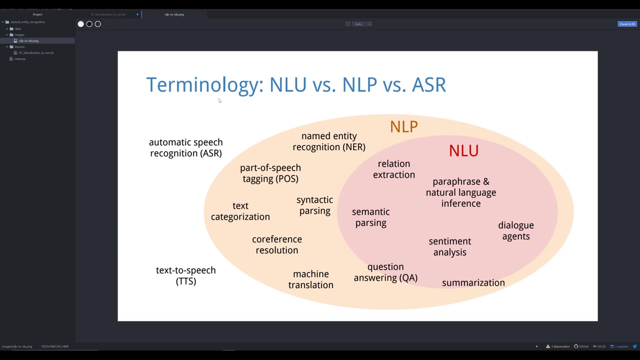 that you're going to need to know. going forward are is natural language processing. So natural language processing is a field of artificial intelligence and increasingly more and more so. It's the idea of trying to get a computer to understand human speech and human text And NLP. 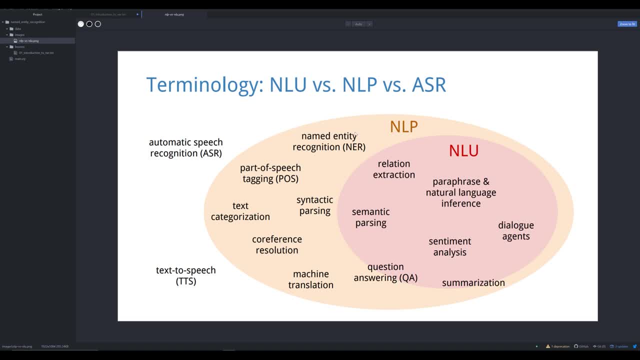 as you can see from this great graph, is oftentimes used in conjunction with NLU, or natural language understanding, and ASR, automatic speech and language processing. NLP is a general field in which you also have natural language understanding, And this is where 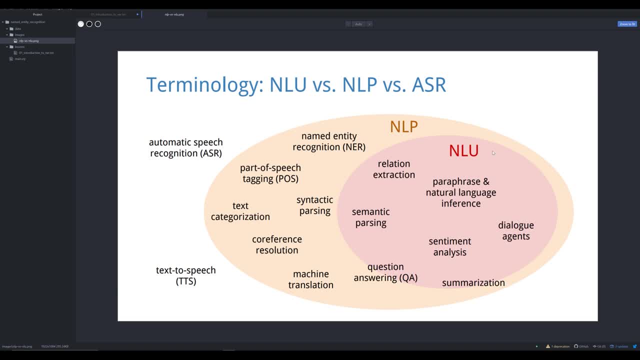 you get things like a computer that can recognize sentiment of a text. So if a movie review is positive or negative, if a post should be flagged as inappropriate, therefore allowing the administrator to see inappropriate texts on their website without having to actually read them. Other things that it's used for is data summarization. so summarizing: 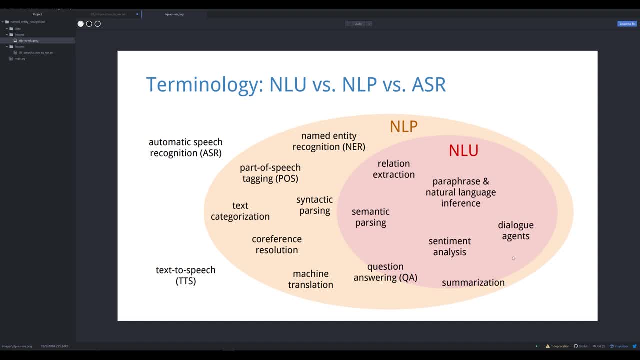 texts. So if you have thousands and thousands of pages and you don't want to read them all, NLU is very useful for telling you what's in those thousands and thousands of pages, pages. It'll give you a few paragraph summary of the text. That's NLU and it falls under this. 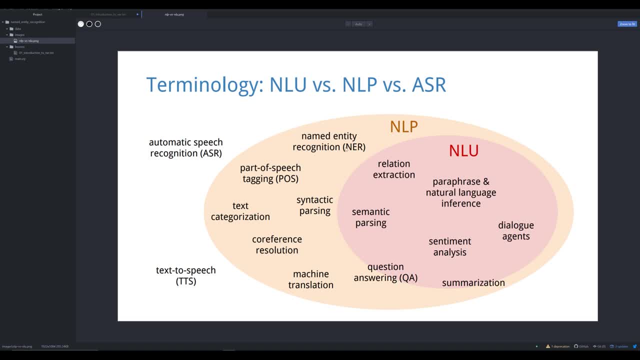 umbrella of NLP And this is where named entity recognition is and this whole strata of natural language processing. It is a technique or a task of natural language processing. It is the process by which we take a text, feed it to a computer and extract a series of structured data from that. 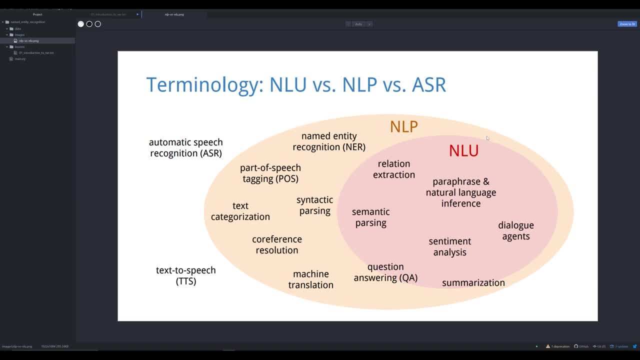 text. Now named entities can be anything from a date to a person's name, to a particular location. NER is the process in which we extract that metadata from a text so that we can identify patterns in texts without having to read them. So when is this useful? Well, it's useful for: 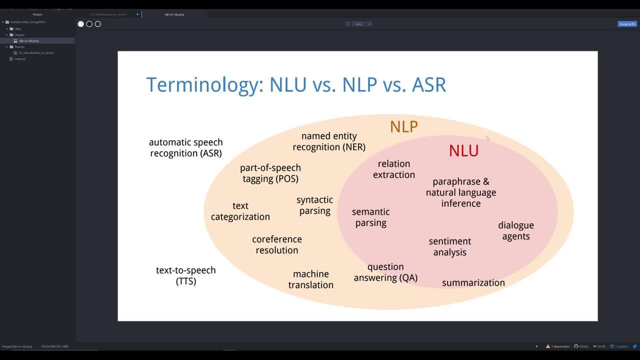 scholars who have millions of pages of text that they cannot physically read in a single lifetime, much less the few months of reading time needed to cultivate a pretty good workflow for a scholarly paper or article, or the years it might take to write a scholarly book. So what do you do in these scenarios? Well, you automate. 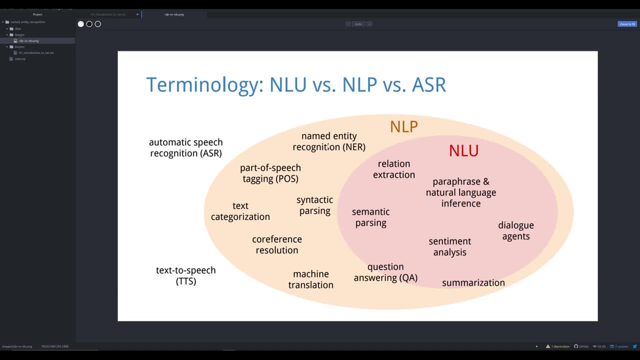 certain tasks, and we can do this through natural language processing, and we can do this through specifically named entity recognition, which allows for a researcher to identify and target texts to look at more closely, or to extract names and entities from a bunch of texts to. 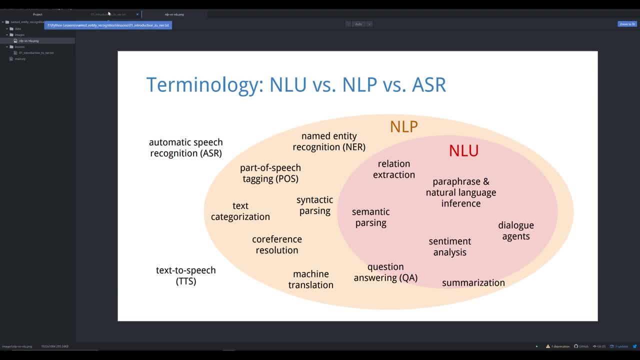 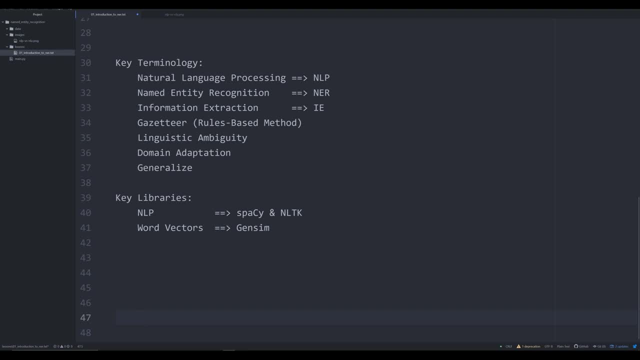 do distance reading. So that's kind of the general purpose of named entity recognition and where it fits into the overall umbrella of natural language processing. So this is part of a process that we call information extraction, ie so extracting information from a text to store it as structured. 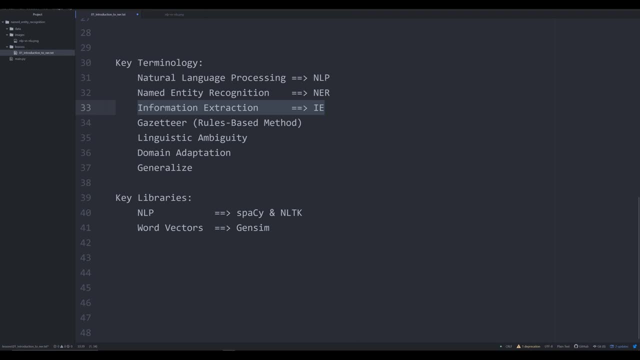 data. Now, there's really kind of two different ways to do this. There is a machine learning approach, which is what this entire series is going to kind of focus on, And then there's a tool that we're going to focus on, And there's also a gazetteer or a rules based method. a gazetteer- 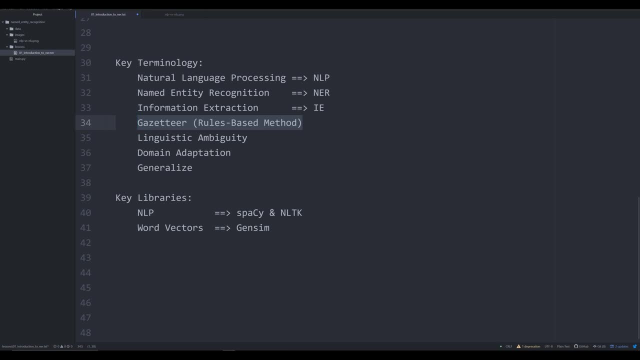 I'm going to talk about more in the next video, But it is essentially a dictionary, a list of types of named entities that fall under a specific category. So if you had a list of people's names, you would just go across an entire text And if a word that is found in that text matches a name that is in a 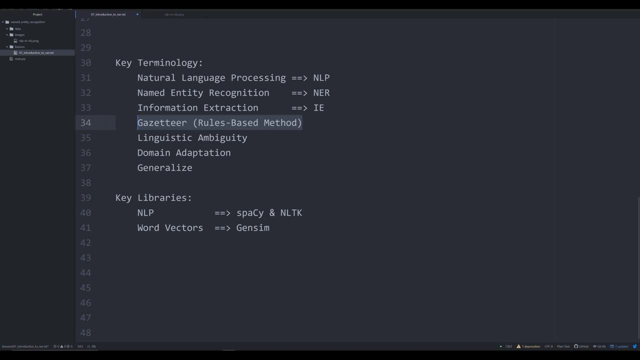 list of names that you've got stored somewhere else. this gazetteer will flag it and tag it and it will mark it as a named entity, specifically a person, as we are going to see. that is very useful for certain applications, But it has a noticeable weakness that we're going. 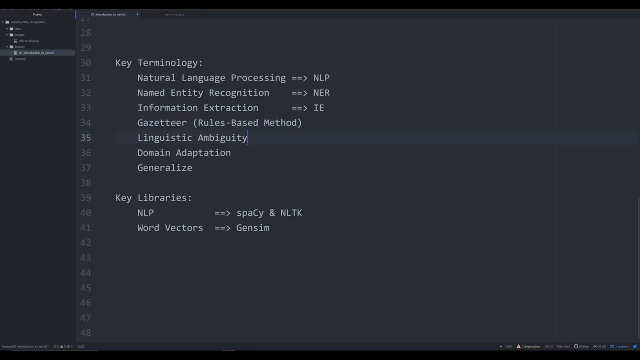 to talk about in the next video. The reason why natural language processing is such a difficult task, and named entity recognition even more so, is because of what we call linguistic ambiguity. So language is naturally ambiguous. It's what makes language beautiful. It's what allows us to write. 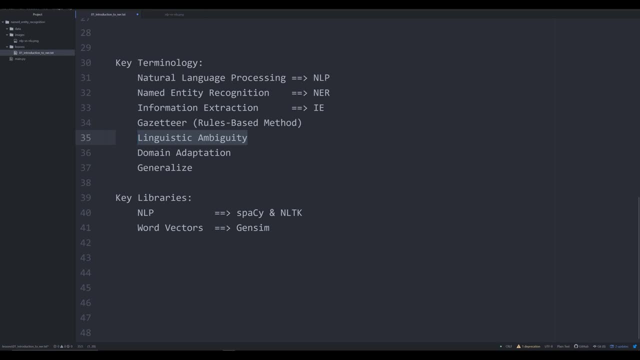 poetry, make jokes that are puns. It's a naturally ambiguous thing that we humans have And it's what causes confusion and difficulty in training a computer to understand human speech. Things that we do without realizing, like taking in the context of a word which we're going to see in the next. 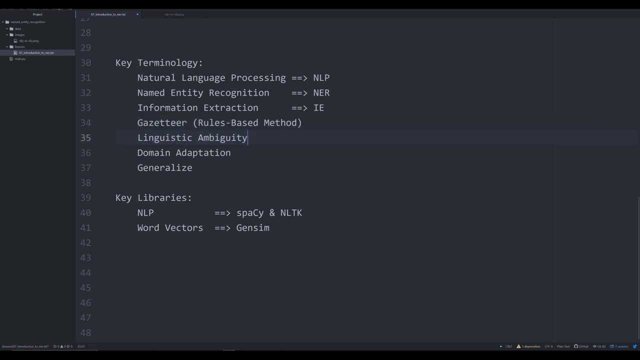 video is actually incredibly difficult for a machine to do without a complex set of algorithms in place, And we're going to see throughout this entire video that there are a lot of things that we're going to be focusing on in this entire series: how linguistic ambiguity is going to be. 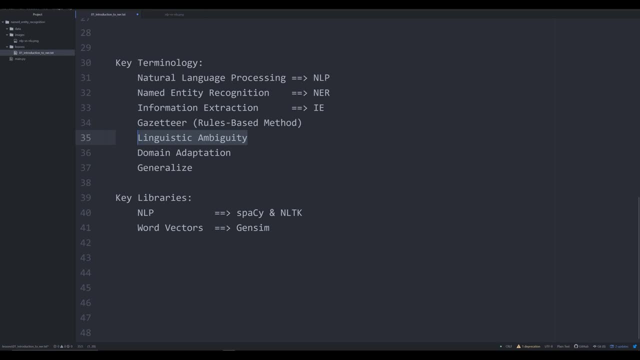 causing us to think about how we approach named entity recognition and approach natural language processing generally, And what I'm really going to focus on in this series is a problem that I haven't really seen explored on YouTube and it's a little difficult to find on the web in general. 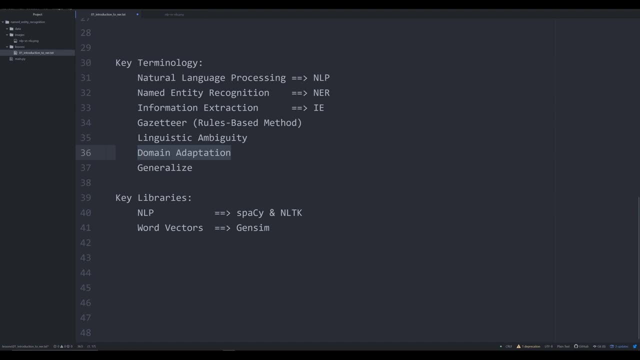 which is something called domain adaptation. This is the process by which we take existing models and we adapt them to a specific domain. Now, in this series, I'm going to be talking about doing domain adaptation with Holocaust specific data. So how do you get a model that has never really? 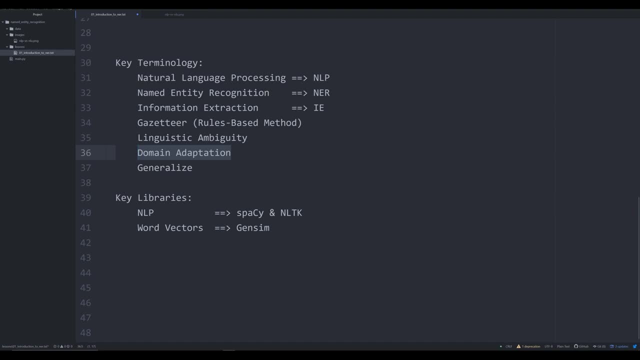 encountered Holocaust documents familiar to some degree, with textual data that might be relevant to the Holocaust, And so that's what we're going to be talking about in this series, And if you take the methods I talk about in this series, you can apply them to any domain. The methods I'll 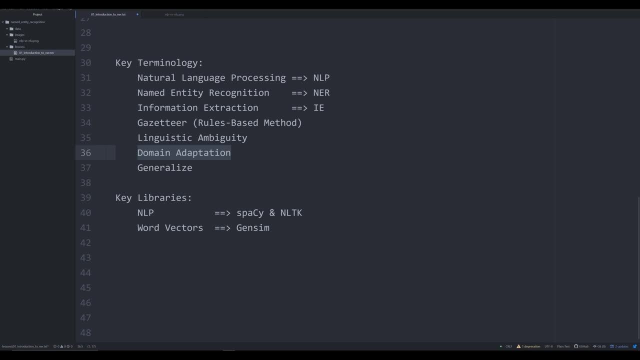 show you will be the methods I use to apply them to any domain. So I'm going to be talking about the methods I use to apply them to any domain. So I'm going to be talking about fairly easy to modify and adjust by just using different corpora of texts that are specific to. 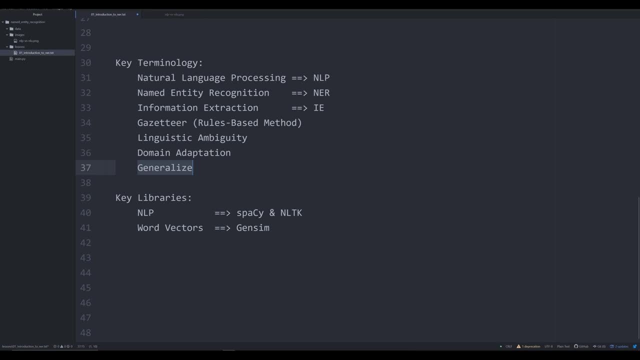 your research. The other thing that we should be familiar with is this idea of generalize. This is something that is a common element of machine learning. You want to produce models that can generalize well. What is generalization? Generalization is the ability for a model to perform well on data that it has never seen before. 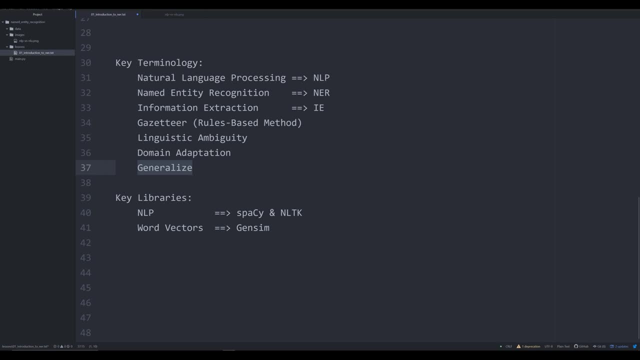 So you cannot possibly give a machine learning model every single thing that has ever been written by mankind. It would be too large. In fact, somebody actually has done this. Those over at OpenAI have produced- you might have heard about it- GPT-2 and now GPT-3,. 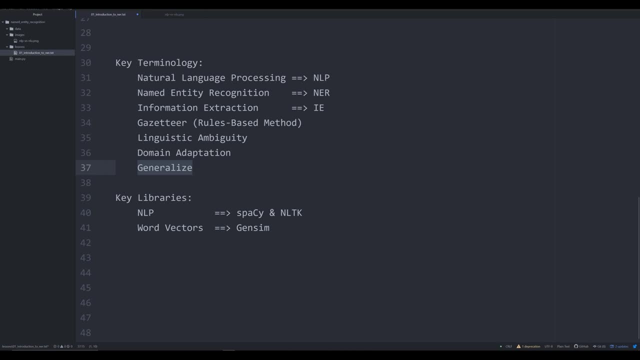 which were trained on an immense corpus the likes of which no other model has ever been trained on before, And the size is so large with GPT-3 that it cannot be run on a local machine. And the result of this is that the models are not immediately a level before the model in a real context. 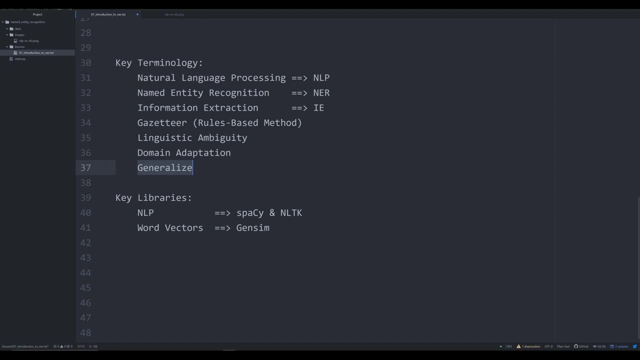 It's not just a globalization model, It's actually a humanized model, It's a state of the art type of model, And so this is the idea of creating a mode of that kind of model that allows for the models to produce state of the art, human-like intelligence. 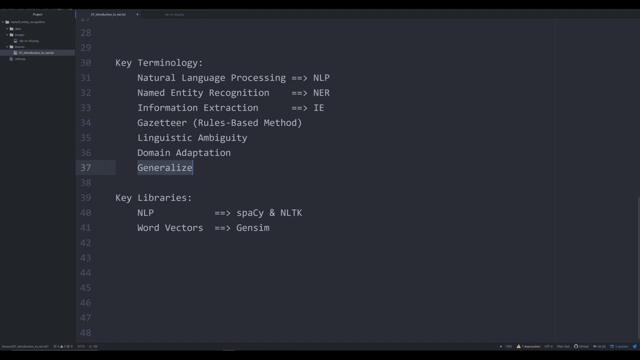 with understanding of text and generating text with very little to go on. A little difficult to explain, not going to get into it in this video, But generalization is the ability for the model to essentially generalize and assign named entities, in our case to texts that it has never seen before. And this is the goal of any machine learning, NER model And, like a lot of machine learning models in the world, there's no model as well. 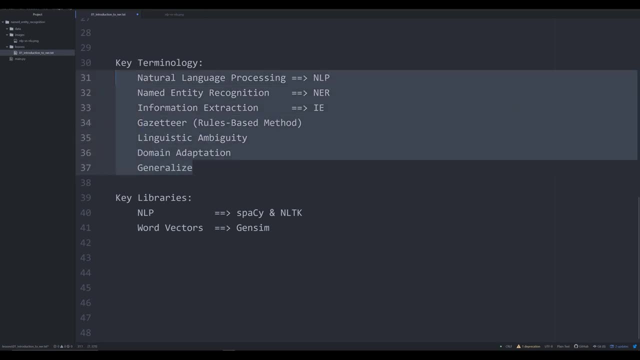 I said during the course of this series, you're not going to have to know the intricacies of machine learning, You're not going to have to learn all the concepts, but you're going to be able to use the power of machine learning, And that's because of the ease of use of machine. 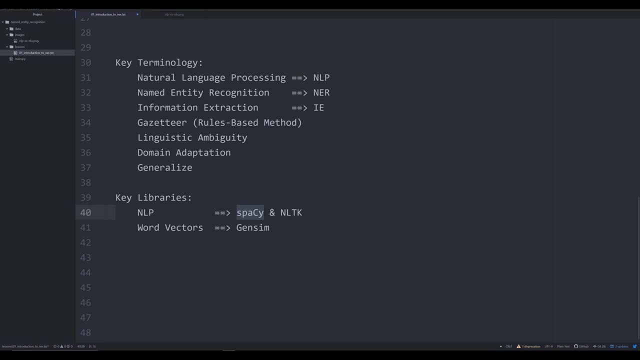 learning libraries in Python, specifically spaCy. Now, if you're performing NLP, you are probably going to be using one of two libraries in Python. You're going to be using spaCy or NLTK, the Natural Language Toolkit. The Natural Language Toolkit NLTK comes out of Stanford and it's 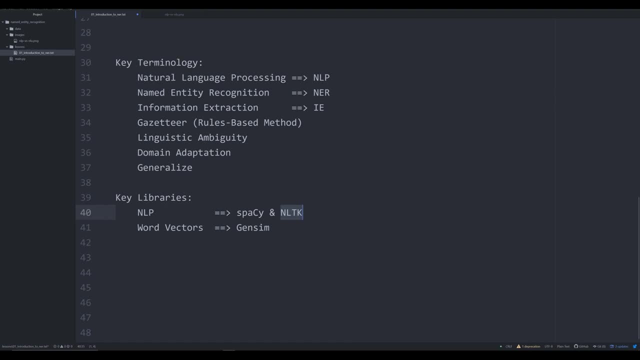 really kind of the standard in academia. It's got some problems. however, The main criticism of NLTK is the speed at which it processes texts. It takes a long time And this is where spaCy comes in. spaCy is a commercial NLP. It's used for more big business tasks, big data tasks, And the reason. 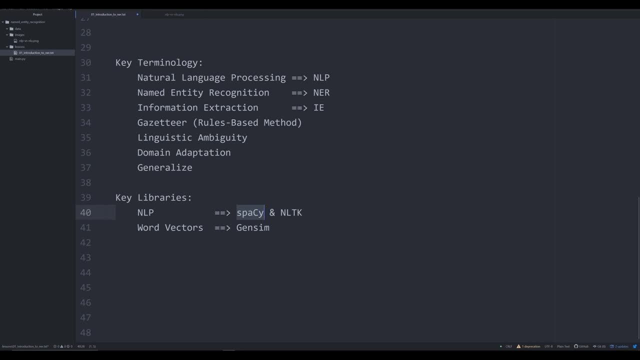 for this is because it has a high accuracy rating. with off-the-shelf models, It's really good at parsing texts and tagging texts And if you're using standard non-domain specific data, it's really good at NER- off-the-shelf- Really good. The reason why people 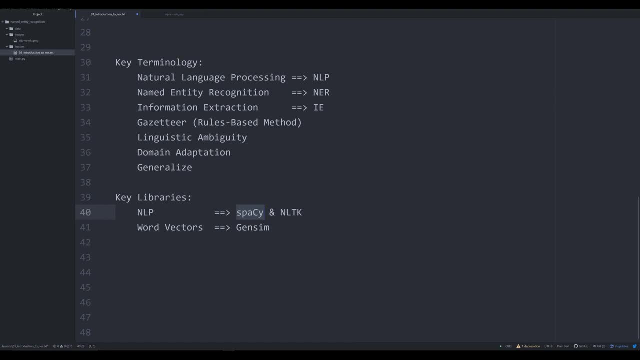 in the commercial world tend to use spaCy and not NLTK is because it scales well. It's really really good at doing a lot of different tasks very, very quickly and efficiently, And in big business you need stuff that can work efficiently and quickly, And the other library that we're 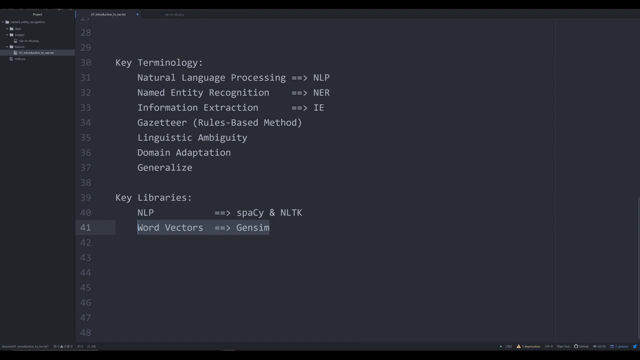 going to be using is the NLP, And it's really good at doing a lot of different tasks very, very quickly and efficiently. And the other library that we're going to be working with in this series is going to be a library called Gensim. Now, Gensim was originally designed for topic modeling, So 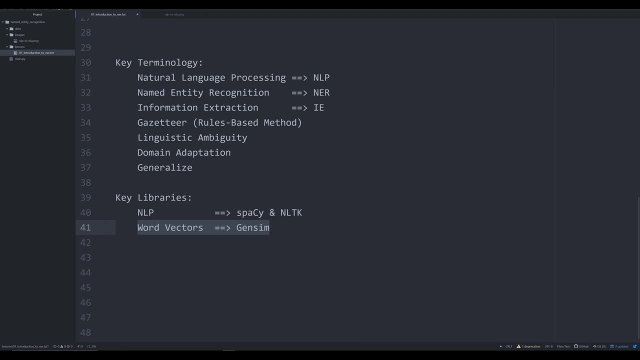 identifying topics in a collection of texts or the topic of a single text. However, in order to perform that task, Gensim had to develop a system by which users could train what we call word vectors. I'm going to be talking about word vectors- a whole bunch, And I think it's video. 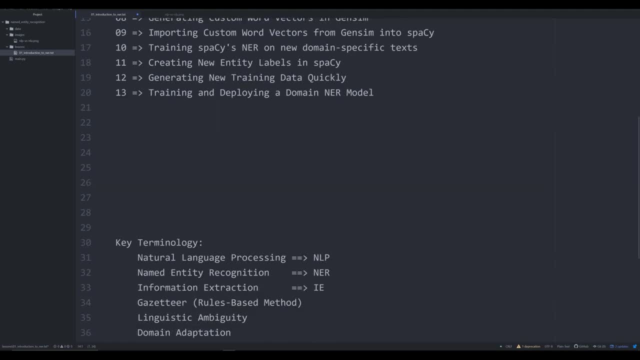 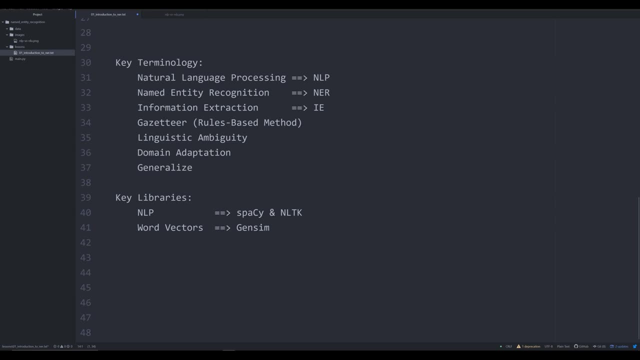 number seven right here, And so if you want to jump ahead, jump ahead to that video, if it's already complete by the time you're watching this. But Gensim is very good and very efficient at training these word vectors, And we're going. 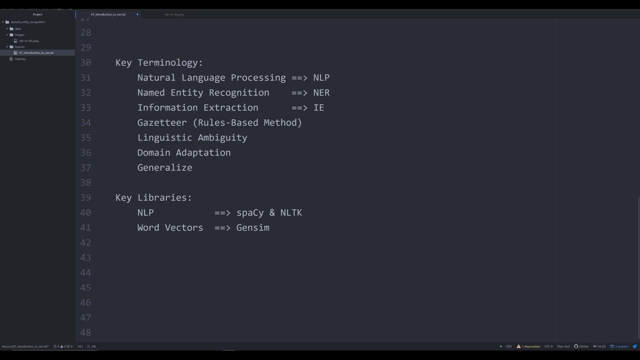 to be using word vectors a lot in this series And we're going to be using Gensim specifically to generate word vectors on a giant corpus of domain specific texts and then injecting those word vectors into spaCy to kind of take advantage of the best of both libraries. This might sound. 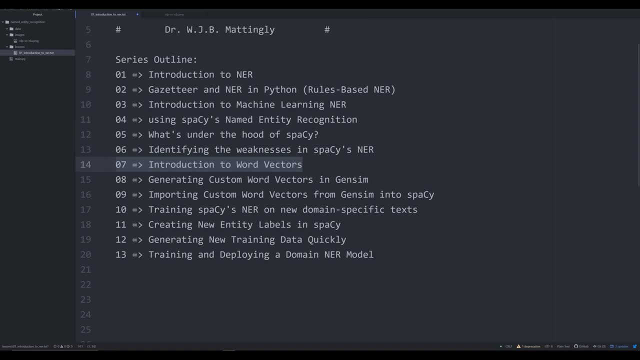 complicated, But if you follow me through this video series, each of these steps, take your time with them. I think you're going to find that the process isn't as scary and as daunting as it might seem. So that's the task before us. Hopefully this sounds fun to everybody. If you have some.